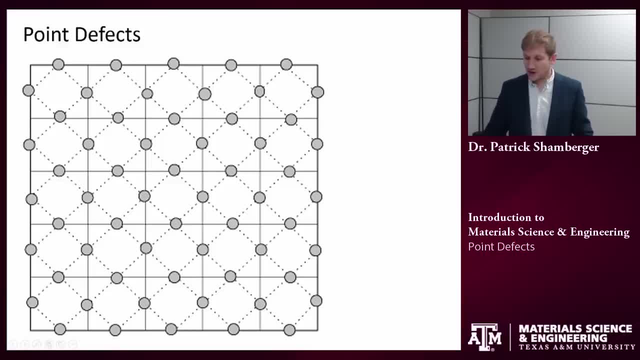 The first is called a vacancy. So if this is our lattice here, if one of these atoms was missing, it's not there. that is what we call a vacancy. Now I'm going to show you the notation for these different kinds of defects as well. 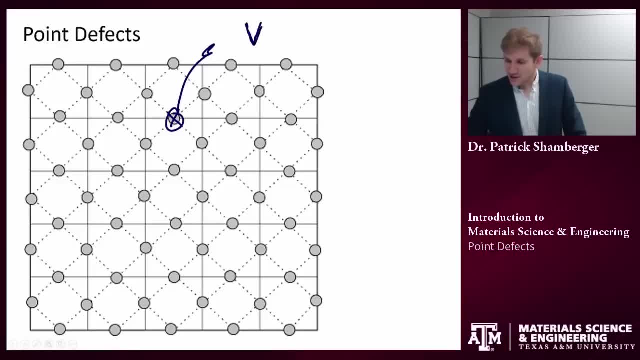 So if we have a vacancy, we symbolize that V for vacancy. then we say what the atom was that is missing, so it was on an aluminum site. say so this aluminum site is gone and then we give a symbol that refers to the charge of this point defect. So in this case, 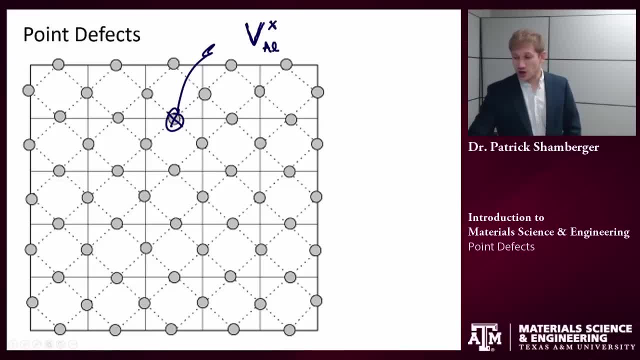 aluminum vacancy and aluminum lattice is a neutral charge, so we put an X there. So vacancy is the first type. The second type would be an interstitial, and that is if we have some other atom sitting in a site in this lattice that is not normally occupied. So let's say 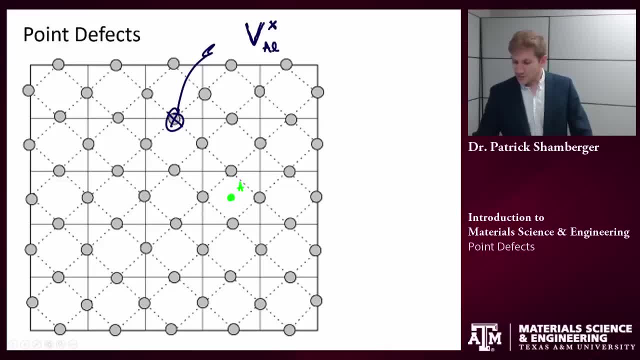 for example, this is still an aluminum atom. I'll say aluminum there. We would notate this. So this is now an aluminum atom and it's on an interstitial site. that's what the I means. and again, it's a neutral charge. So we give a neutral sign. that's the X symbol. 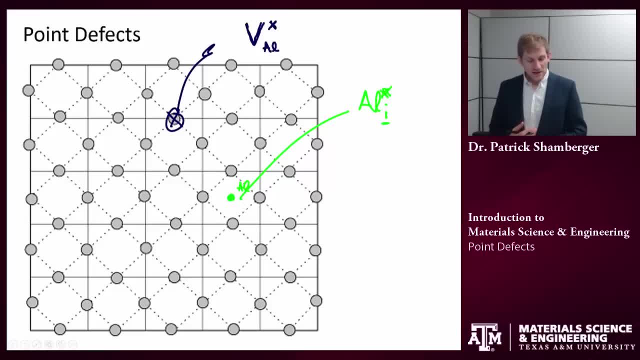 up there. The third kind of point defect that we would see would be a substitute. So if we have a substitution, So again let's say this is a lattice of aluminum atoms, but this atom here is not aluminum. Let's say this is copper. So the notation for this is going to be written. 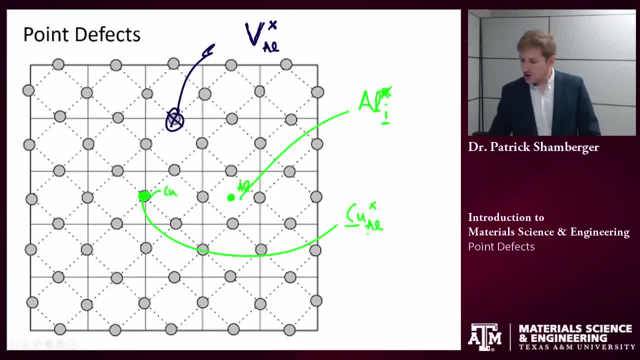 as such. So again, a copper atom is sitting on an aluminum site and the net charge is neutral. So these are the three different kinds of vacancies, of point defects. We have vacancies, we have interstitials and we have substitutions. 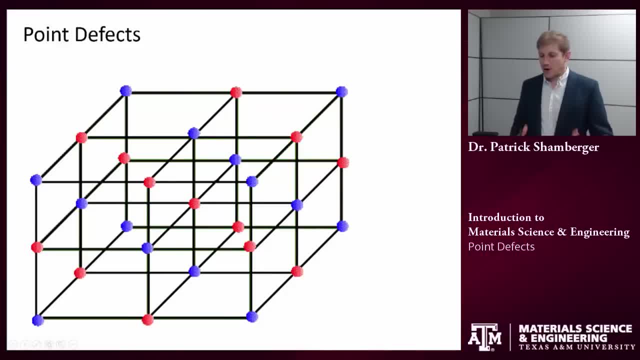 Okay, next we're going to think about ceramic or ionic compounds, And there are additional things that we have to consider in these cases. And that's just because an ionic compound has positively charged ions and negatively charged ions. So let's say, each of these blue. 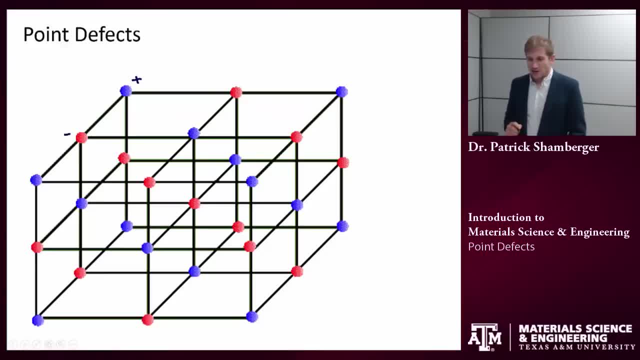 is a cation and each of the red is an anion. And for the purpose of this, let's say, the two of these blue are magnesium, so it's actually plus two, And the red are oxygen, so it's minus two. 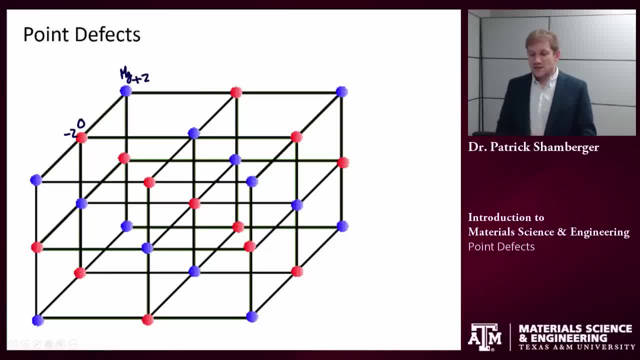 So in the ionic case we can't simply have a vacancy of one of these atoms, because that would lead to a charge imbalance in the system. Similarly, we can't just have a substitution of one other charged species in the lattice, because that would also lead to a charge imbalance. 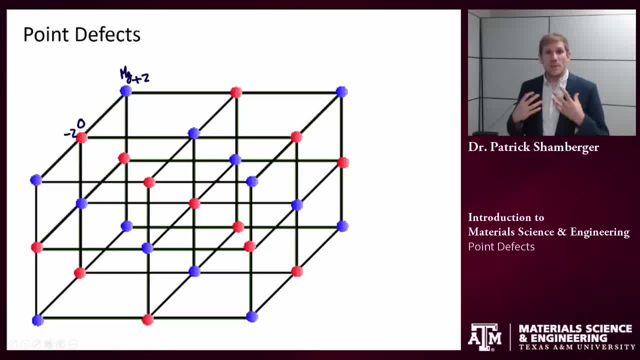 So the rule is that when we're dealing with ionic compounds we always need to maintain charge balance. Because of that, there are two special kinds of point defects that we see very frequently in ionic systems. The first are called Schottky defects And 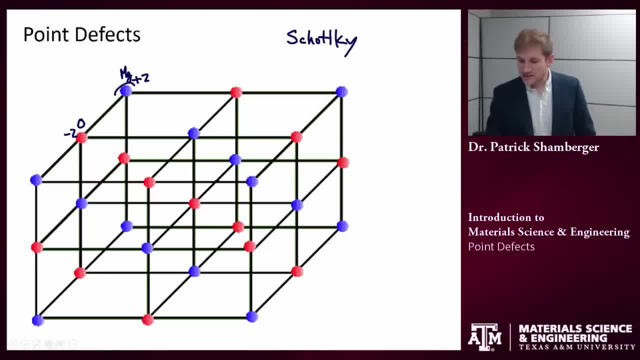 this is when we have a paired vacancy. So let's say, both this magnesium and this oxygen atom are missing. So we're missing a plus two charge and we're missing a minus two charge. So we need to maintain charge balance, The notation for this. I'm going to write it first and then I'll explain what it means. 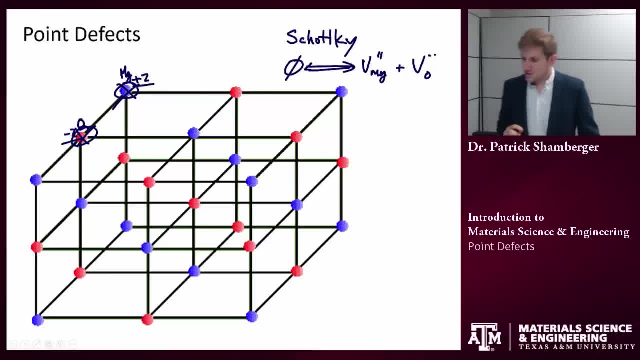 OK, So I've written it like a reaction. So initially we have the pure lattice, But we went to the case where we have a vacancy of a magnesium cation and a vacancy of a magnesium And we have a positive charge of an oxygen anion. Now you'll notice I didn't put an 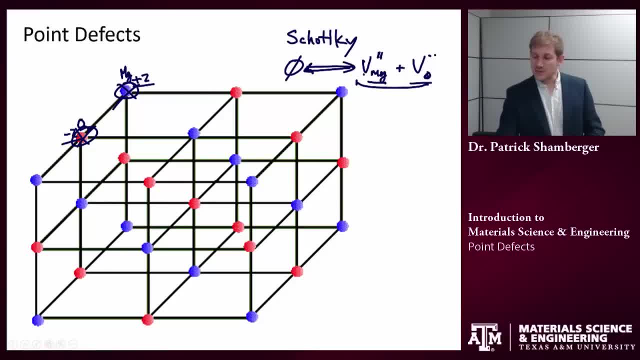 x up here because both of these are charged species. Magnesium has a plus two charge. So if we have a magnesium vacancy that means we have a negative two charge, because that positive two that is usually there is not there. So negative two charge is written by. 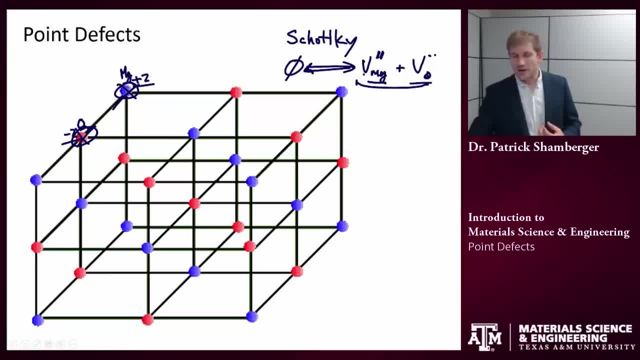 two dashes up here. Similarly, a vacancy of an oxygen would have two positive charge- So we notate that- by two dots up here. So this would be a single magnesium vacancy, a single oxygen vacancy. But again the Schottky defect is where we have the case of the paired vacancies.